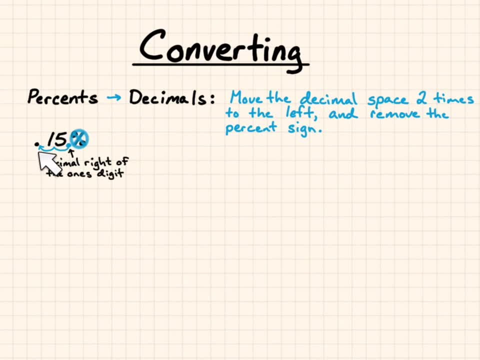 and remove the percent sign For 15%, we end up with 0.15 or we write that as 0.15.. Try these out. 1% and 140%. We put the decimal place to the right of the ones digit and move it twice. 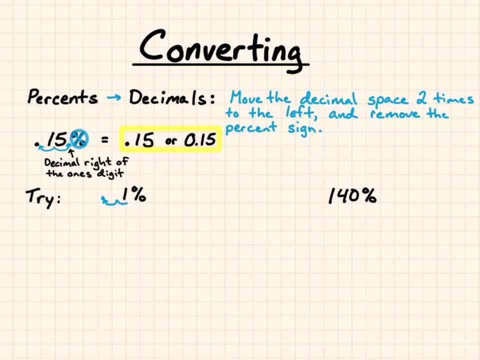 For 1%, there's a void, so we fill it with a zero. You end up with 0.01 or 0.01.. For 140%, you move the decimal place twice to the left and you end up with 0.01.. 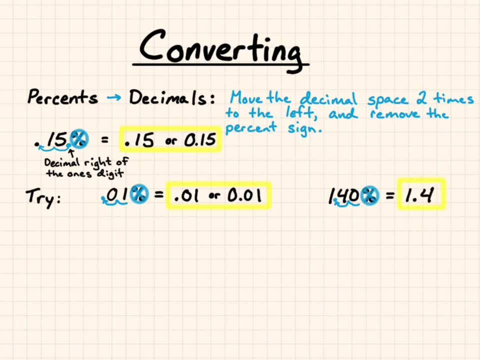 For 140%, you move the decimal place twice to the left and you end up with 0.01.. For 140% you have 1.4.. Converting from decimals to percents, move the decimal two times to the right and add the percent sign. 0.25 becomes 25%. Try these 0.1 and 1.08.. 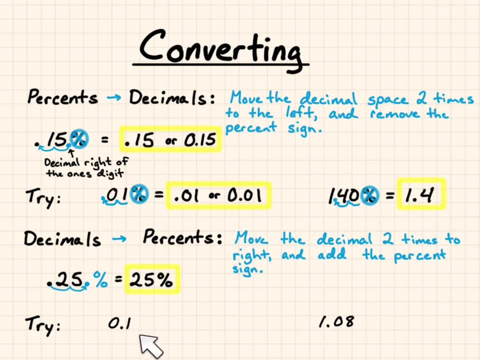 0.1,. I'm going to move the decimal place twice to the right. I have a void right here and I'm adding 0.01.. Then you add the percent sign. You get 10% For 1.08,. move the decimal place twice to the right and add the percent sign at 108%. 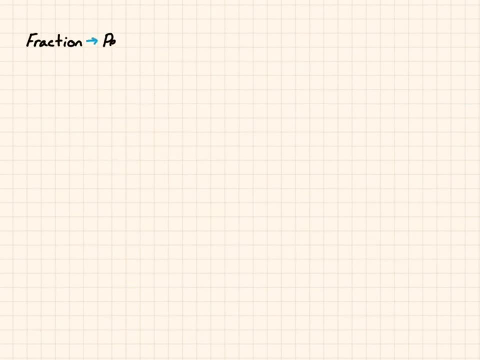 Next topic is fractions to percents. For 0.14 change fraction to decimal using long division, The bottom goes outside, the top number goes inside. four doesn't go into one. you add a decimal and bring it up and then add a zero. one point zero is the same as one or it has the same value of one. but i can see how many times. 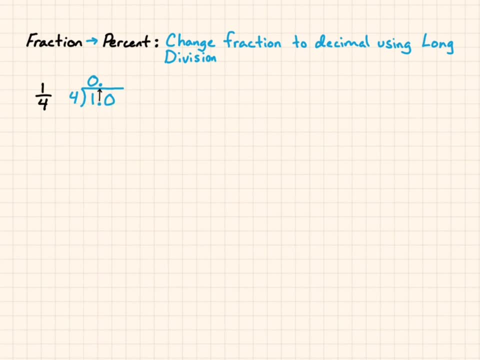 four goes into ten. ten goes. four goes into ten two times two times four is eight. i subtract, i get two as a remainder. i still have remainder, so i'm gonna add another zero and bring it down. four goes into twenty five times. five times four is twenty. i subtract, i get zero, so one.